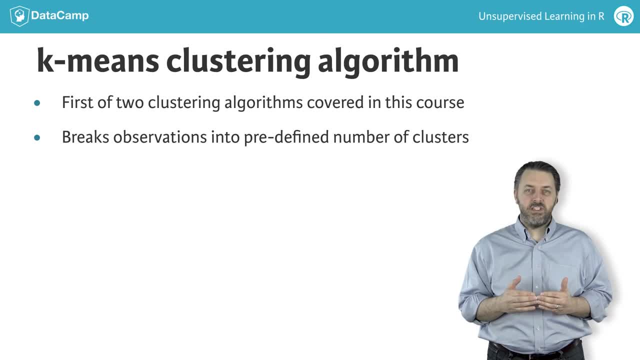 In the next video we will go deeper into how the K-Means algorithm works to achieve this goal. For example, one might hypothesize that this data shown on the screen contains two subgroups. The K-Means algorithm would assign all points in the top right-hand corner. 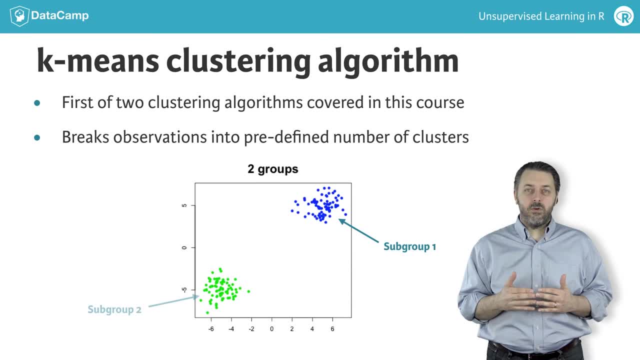 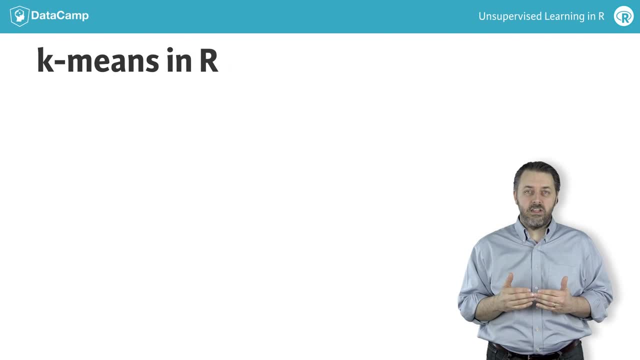 to one subgroup and all observations in the bottom left-hand corner to the other subgroup. K-Means in R comes with the base R install. Invoking K-Means in R is simply a function call to the K-Means function, typically with three parameters. 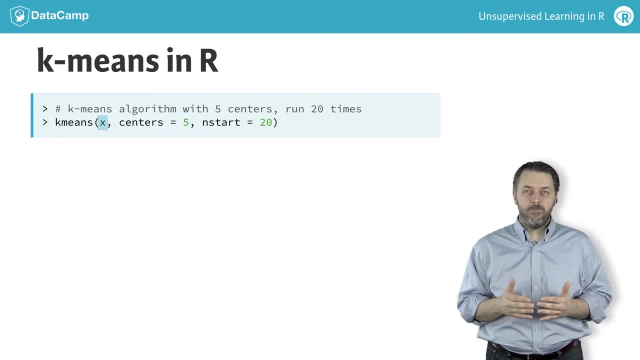 The first parameter is the data represented as x here In K-Means. like many machine learning algorithms, the data is structured in a matrix, with one observation per row of the matrix and one feature in each column of the matrix. The next parameter for K-Means is the number. 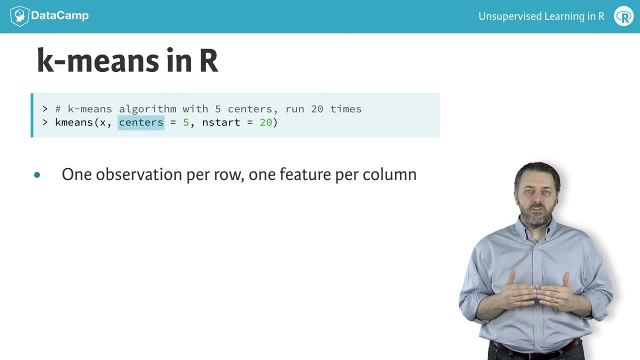 of predetermined groups or clusters. This parameter is called centers, for reasons that will be covered in the next video. Finally, the K-Means algorithm has a random component. The implication of this stochastic component is that a single run of K-Means may not find the optimal solution to K-Means. 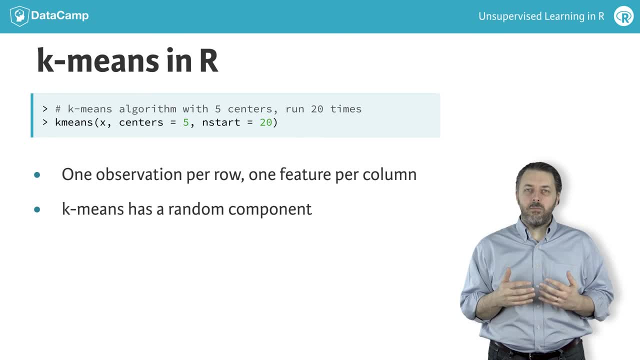 To overcome the random component of the algorithm. K-Means can be run multiple times, with the best outcome across all runs being selected as a single outcome. n-star is the parameter that specifies the number of times K-Means will be repeated. 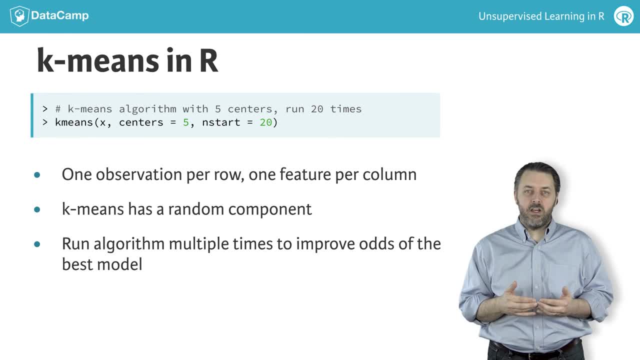 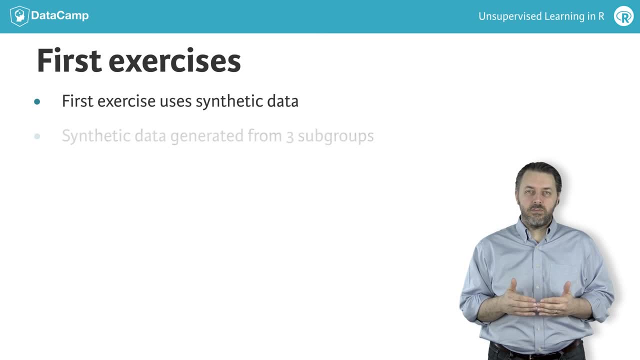 There are other parameters to K-Means and I encourage you to check those out in the R documentation. The first exercises use synthetic data that were generated from three subgroups, but if you plot the data, it might only appear to be two subgroups. Later in this chapter you 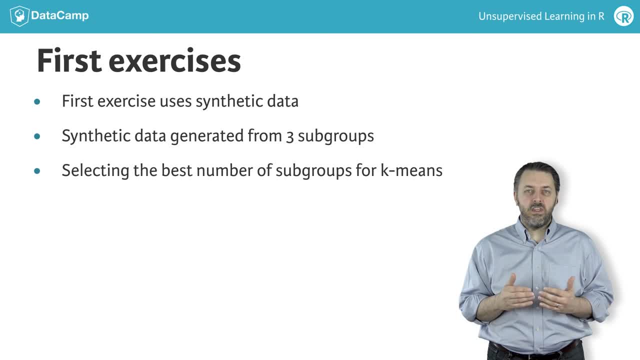 will see how K-Means can be used to estimate the number of subgroups when the number of subgroups is not known a priori. Later in this first chapter of the course you will get experience applying K-Means with a real-world but fun data set. With that information, let's 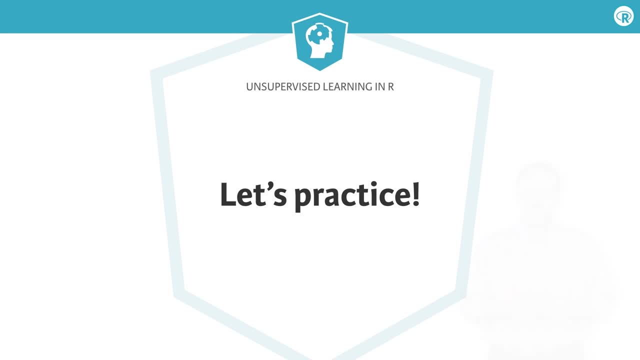